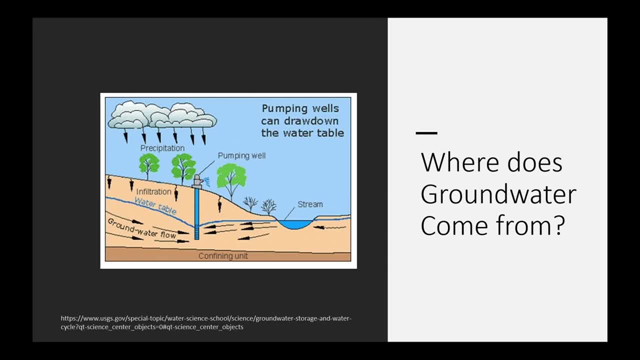 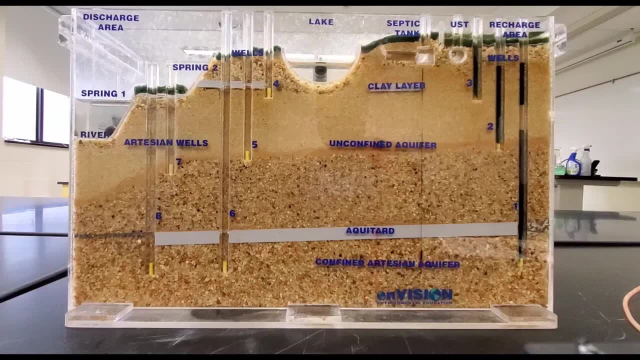 where the soil reaches water capacity and is completely free. Here we created a time lapse of a groundwater model to show you how groundwater contamination and flow work. For this, several different water wells are modeled. There are three types of wells displayed: One in the clay layer, one in the middle where the unconfined sand 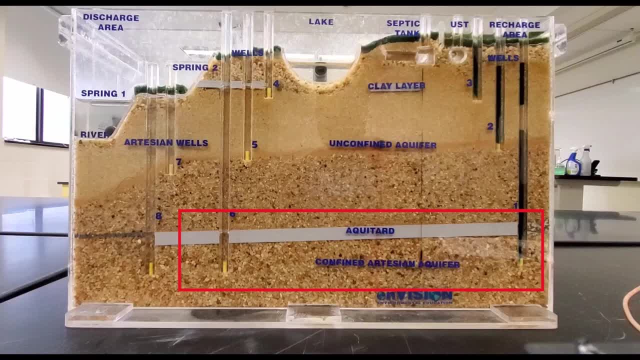 layer is not bordered by an aquitard and another in a confined aquifer which is underneath an aquitard. This model has already had contamination added to the wells on the right side, which is represented by a dark colored dye. Contamination of a well can have several different 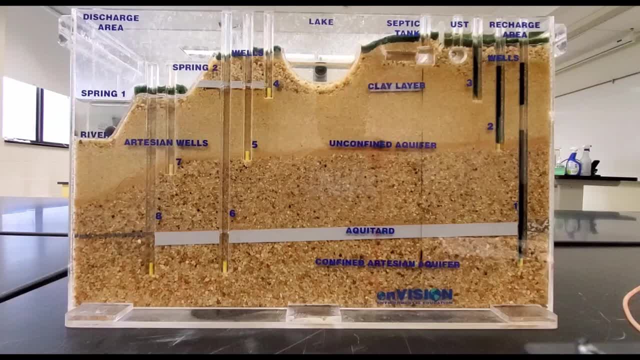 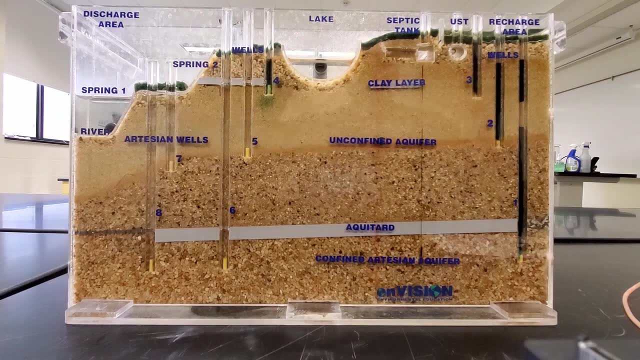 sources, from nearby landfills, septic systems, road salts storage tanks and many others. The model is designed to visualize how groundwater contamination spreads After the dye is added to well 4,. it spreads through the well and into the sediment Because the well is in. 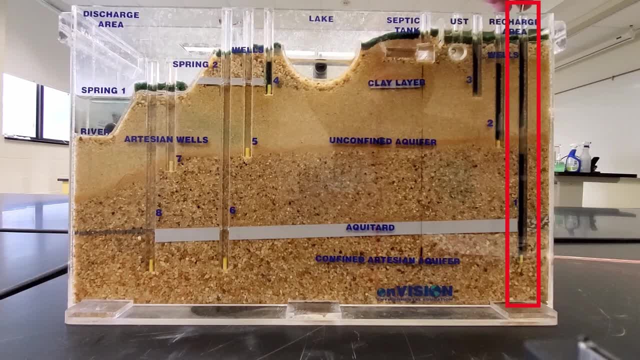 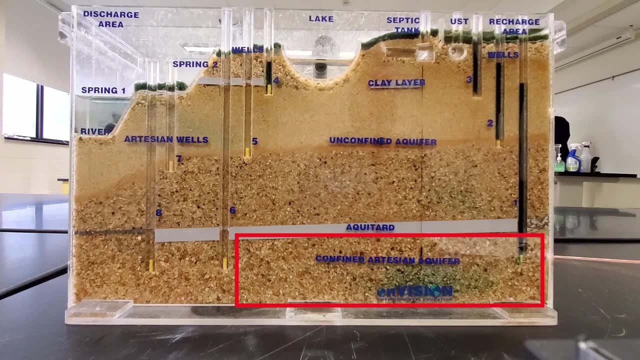 the clay layer, it does not spread very far. When dye is added to well 1,, the dye spreads into the ground beneath the well. In the video you can see that the dye spreads out further and faster than the previous well. This is because of the larger space in well 1, which 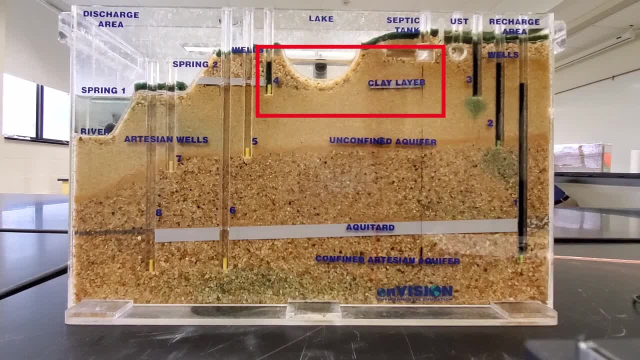 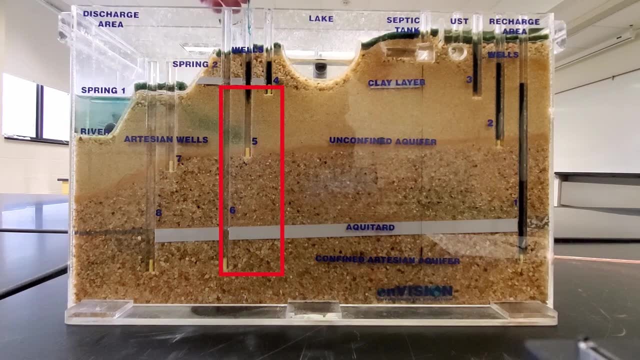 reaches down into the coarse sand layer, whereas well 4 is in the clay layer. Dye added to the 4th and 5th well also spread throughout the wells, though the dye from well 5 does not travel below the aquitard. The dye from all wells travels to the left. 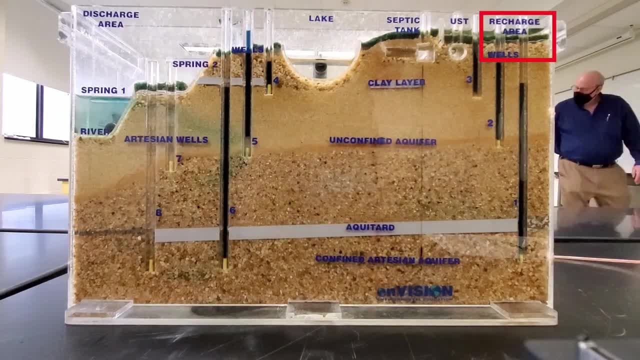 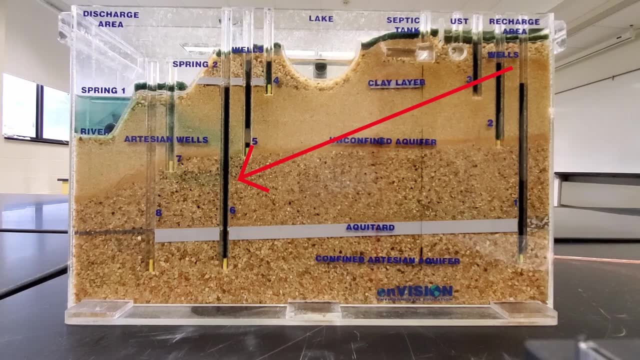 of the diagram. following the flow of water that starts in the upper right corner labeled recharge, It then flows down through to the left side of the model. This creates what is called a hydropower. The water follows along the hydraulic gradient, spreading out of the wells to the left of 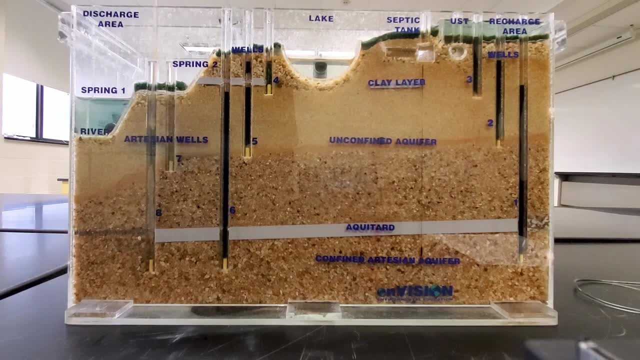 the model. Afterwards, we remove the dye from each of the wells with an eyedropper. Similar processes, along with dispersion techniques and chemical treatments, can be applied to real contamination sites. These endeavors are referred to as groundwater remediation, which we will cover in a later video. 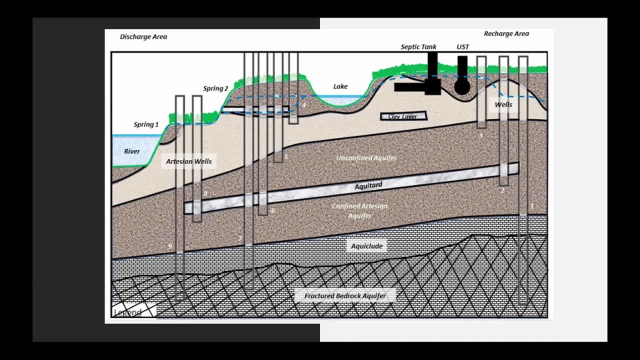 Groundwater is used by millions of people to gain access to clean water and to clean water, and its value as a resource cannot be overstated. Groundwater contamination is a serious matter that can have dangerous, widespread impacts on water quality and accessibility, With extensive remediation efforts statewide, one of the main goals of the triage project.